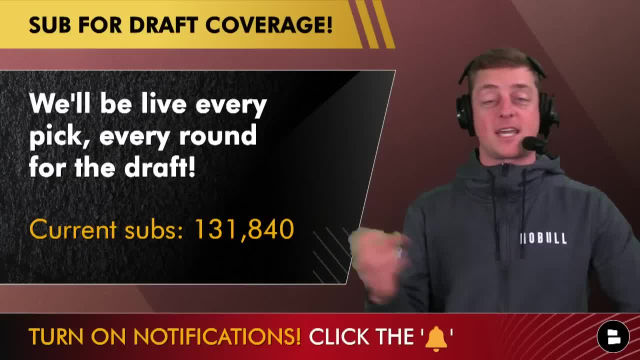 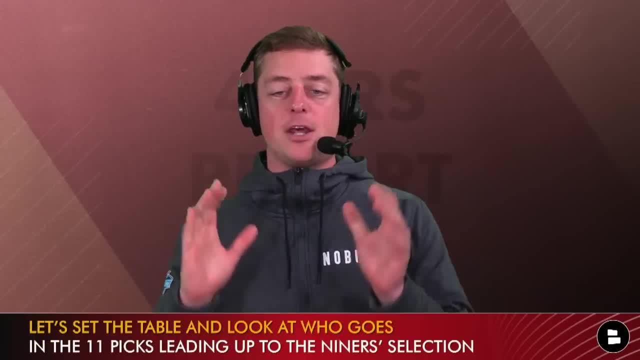 every single round. it's going to be entertaining, It's going to be insightful, It's going to be fun. It's going to be a long weekend, but we're going to spend it together. Let's set the table First and take a look at who goes in the 11 picks prior to the Niners selection, with the 31st overall. 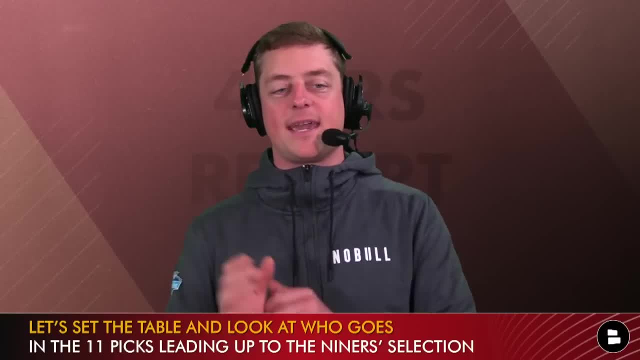 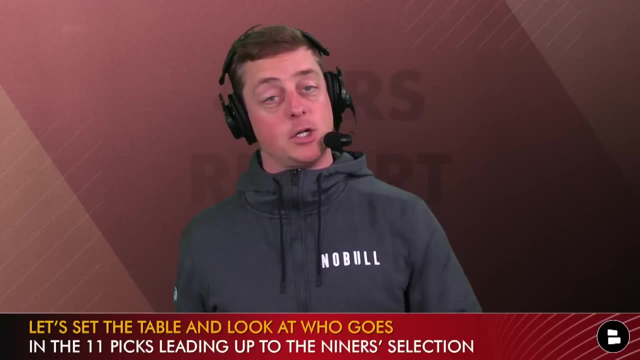 pick, And I think this is good to do because it gives you an indication for which players could be on the board, which players might not be on the board, And a couple of players, obviously, who we've talked about a lot here on the show as potential targets and players of interest for San. 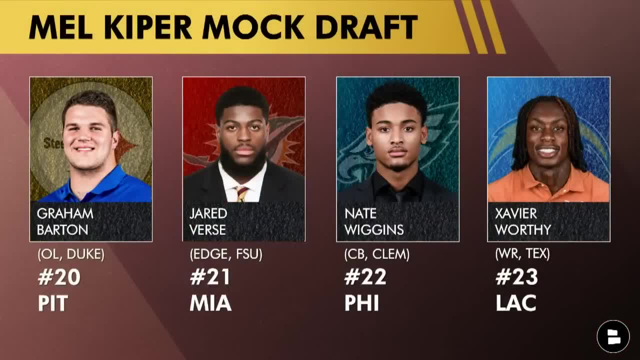 Francisco. So Mel Kuyper has Graham Barton, interior offensive lineman, out of Duke going to the Pittsburgh Steelers, The 20th overall pick. Jared Vers, the second best edge rusher in this class, falling all the way to 21 out of Florida State going to the Miami Dolphins, So he stays in Florida. Nate Wiggins: 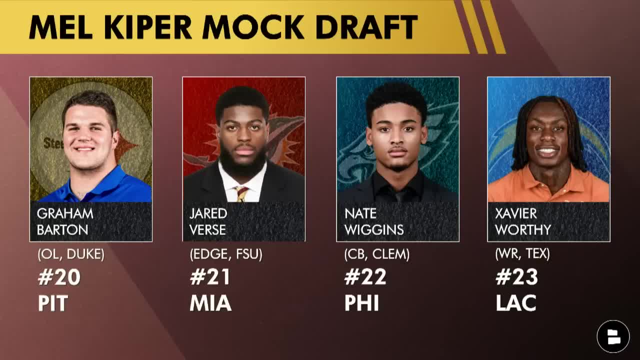 a 4'3" 40-yard dash quarterback out of Clemson going to the Eagles at number 22.. Speaking of fast, nobody's ever been faster than Xavier Worthy out of Texas. At the NFL Combine he ran a 4'2". 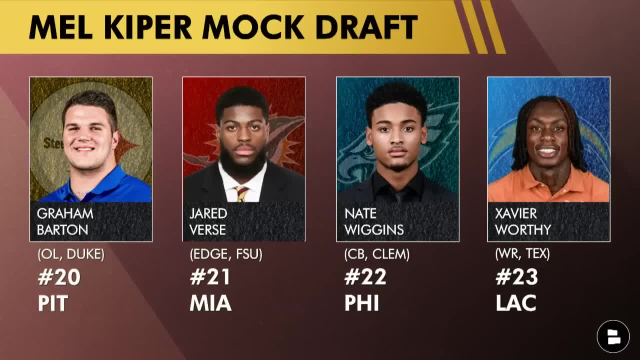 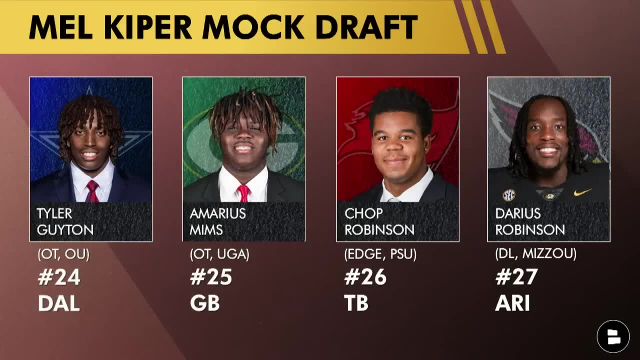 40-yard dash. and now he gets to go play football under Jim Harbaugh, According to Kuyper, with the Los Angeles Chargers, Tyler Guyton going to the offensive lineman needy team in the Dallas Cowboys, not a far trip from Oklahoma, So he goes to the Cowboys. 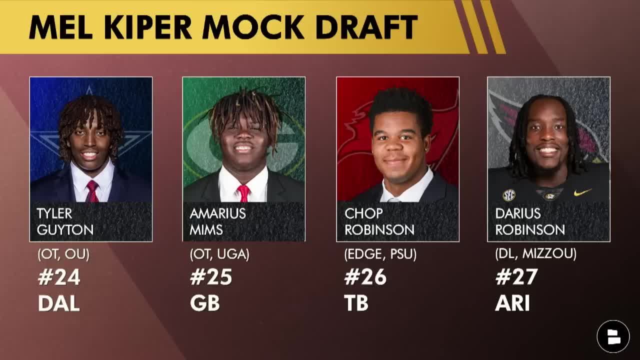 at number 24.. And then another offensive tackle here who's extremely gifted at 6'8", 3'40", only eight college starts, but my goodness does he have a lot of ability. and just a freak athlete, Amarius Mims to the Green Bay Packers at 25th overall, One of my favorites in this. 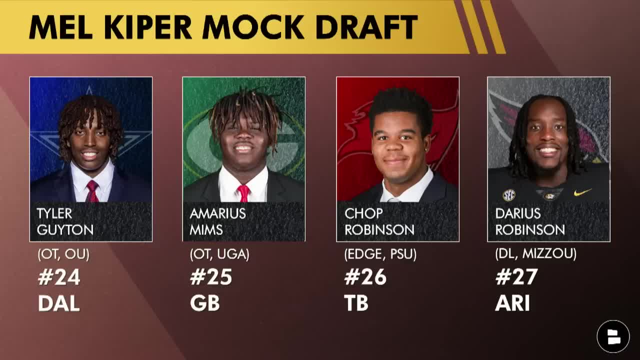 draft is Chop Robinson. I love the fit of him going to the Tampa Bay Buccaneers Defensive-oriented coaching staff. I think they're going to be able to maximize the player, if that rings true. And then back-to-back edge rushers here Darius Robinson, He could play on the edge. 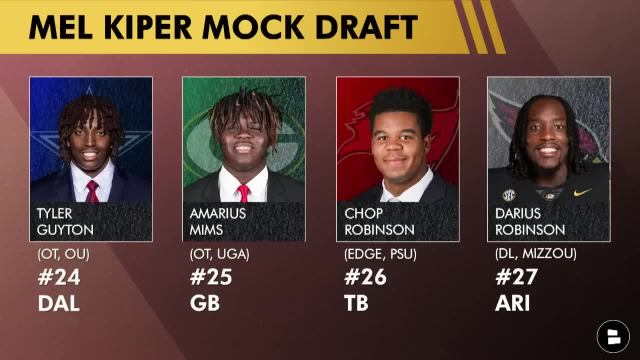 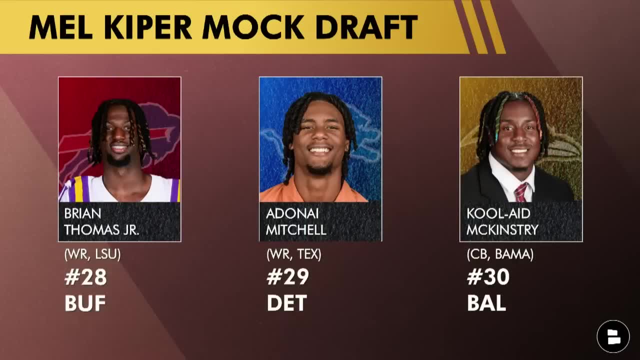 he could play a little bit on the interior Breakout season in 2023. for Mizzou, He goes to the Cardinals with their second selection in this first round. Now things start to get a little bit more interesting. Brian Thomas, wide receiver out of LSU Big with a lot of speed to the Buffalo. 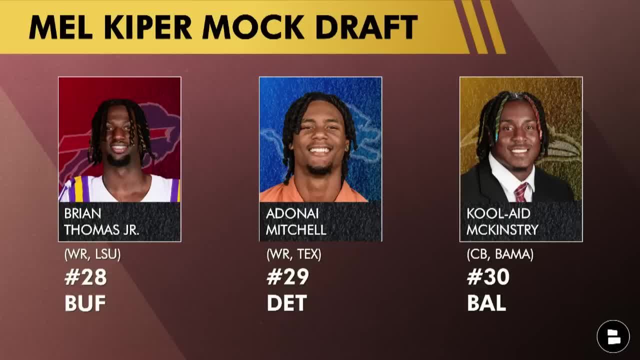 Bills at 28.. They traded away Stephon Diggs and they find the replacement there, AD Mitchell. to the Detroit Lions, Another weapon for that offense, and if that happens it's going to be really scary. 4'3"- 4'4" guy is also built at 6'2", has everything to his route tree And then 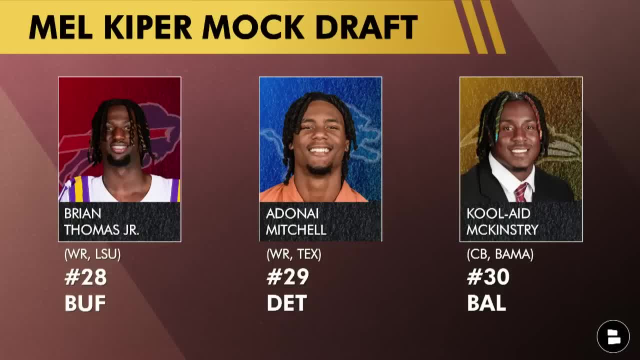 Kool-Aid McKinstry. This is such a Ravens pick because they always like to prioritize defense. Last year had the best defense in the National Football League. he's got swagger. he's a dog. that fits the profile for what the Ravens look for for their 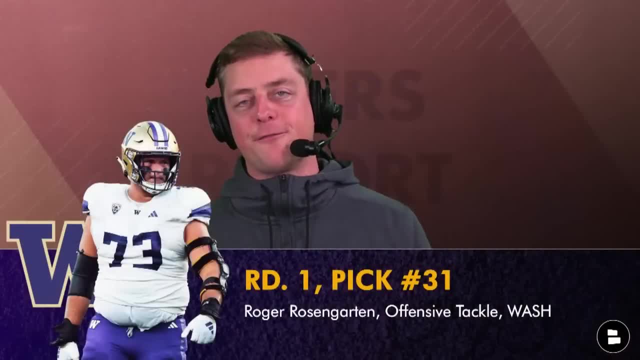 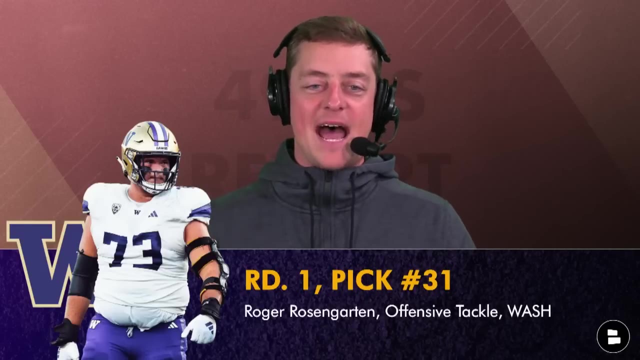 culture. Now the Niners are on the clock: 31st overall pick, second to last selection in the first round, and Mel Kuyper has San Francisco going with Roger Rosengarten Offensive tackle out of Washington. This is the same player who Kuyper had going to the Niners in his first mock. 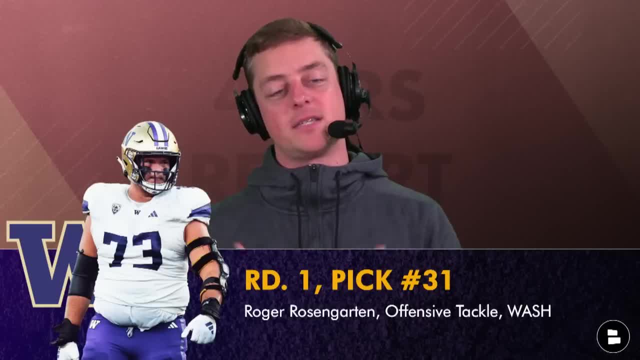 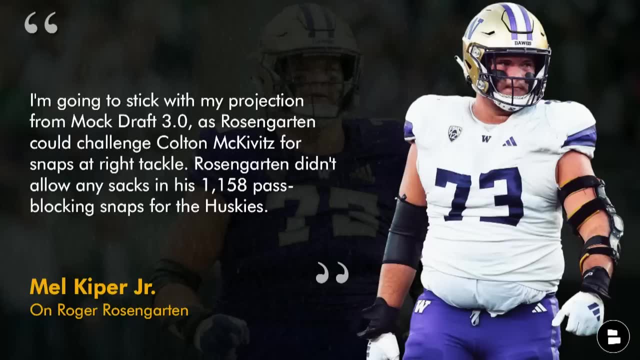 Was he lazy? He didn't want to switch it up. Here's his reasoning. I'm going to stick with my projection from mock draft 3.0. as Rosengarten could challenge Colton McKibbitz for snaps at right tackle, He didn't allow any sacks in his 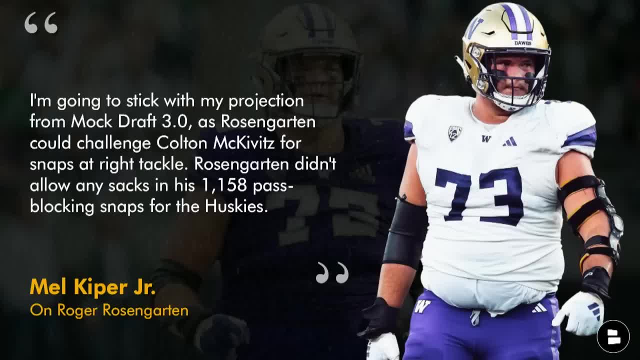 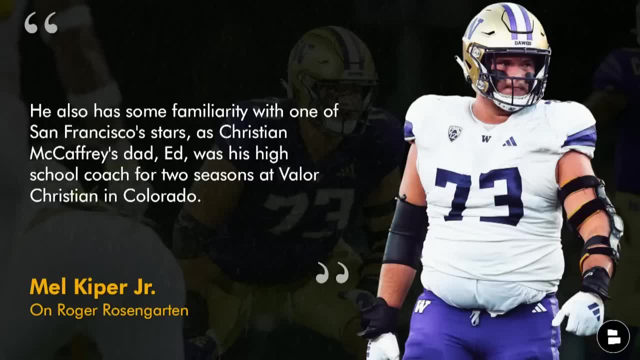 1,158 pass blocking snaps for the Huskies. He also has some familiarity with one of San Francisco's stars, As Christian McCaffrey's dad. Ed McCaffrey, who was an All-Pro, won a couple of Super Bowls. 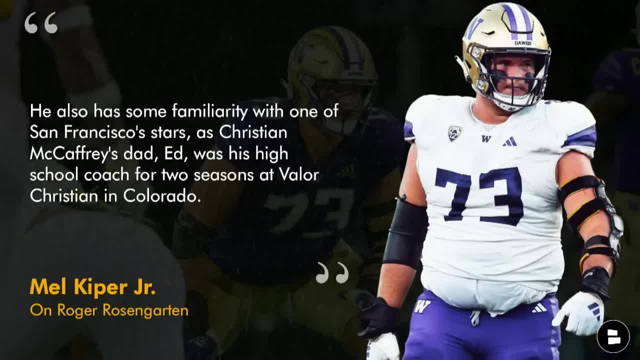 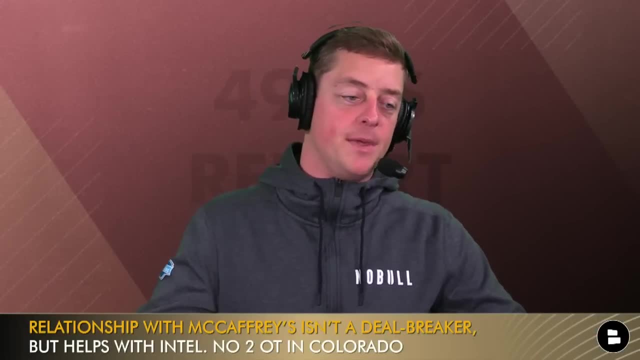 with the Denver Broncos was Rosengarten's high school coach for two years at Valor Christian in Colorado. That's more of an interesting tidbit there. The relationship with the McCaffreys obviously is not a deal breaker, even though Kyle Shanahan loves Christian and grew up being around Ed because Ed was coached. 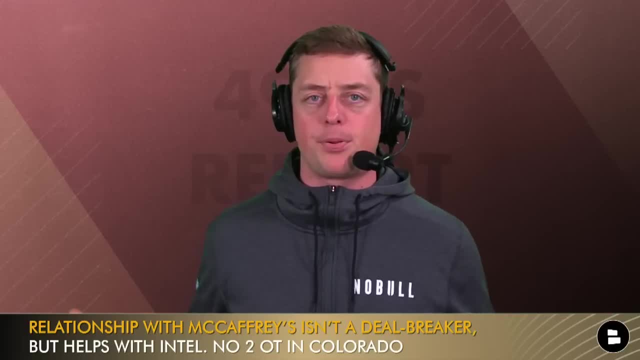 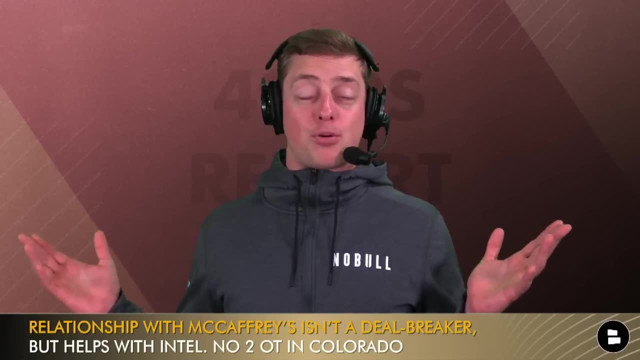 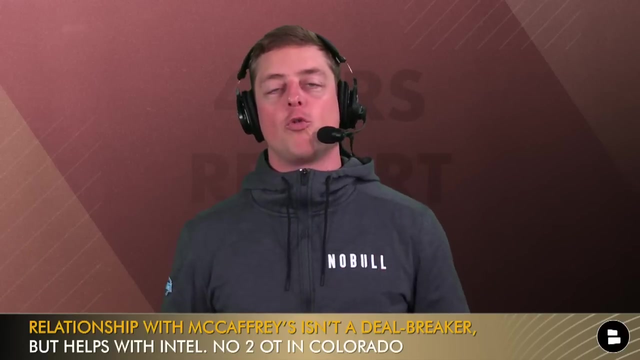 by his father, Mike. But it helps with the intel on the player and it helps you gather some information here. And Rosengarten was the number two overall prospect coming out of the San Francisco State of Colorado. So highly touted high school recruit When I scout him, really good size. 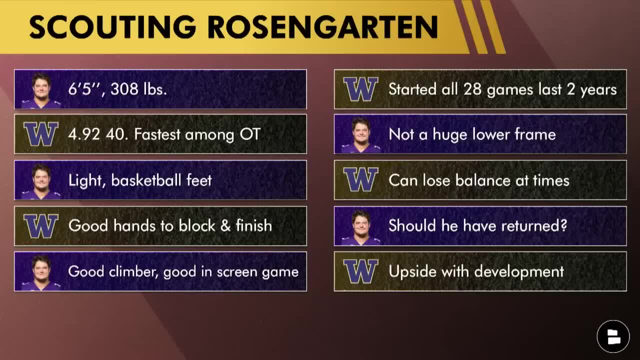 Checks in at 6'5", 308 pounds. He ran a 4'9" 240-yard dash, which is freakish at that size. That was the fastest 40-yard dash among offensive tackles at the NFL Combine. He has light basketball. 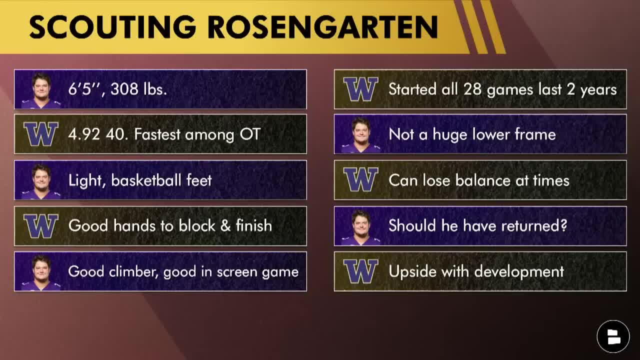 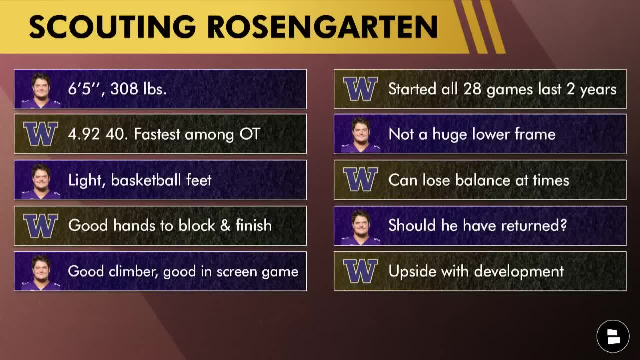 inside. You're usually on the inside. You're usually on the inside. You're usually on the inside. You're getting beat by a fellow defensive lineman. Good hands to block and finish And those hands he's very calculated with how he uses them in his run: blocking and pass, blocking sets. He's a good climber. What I 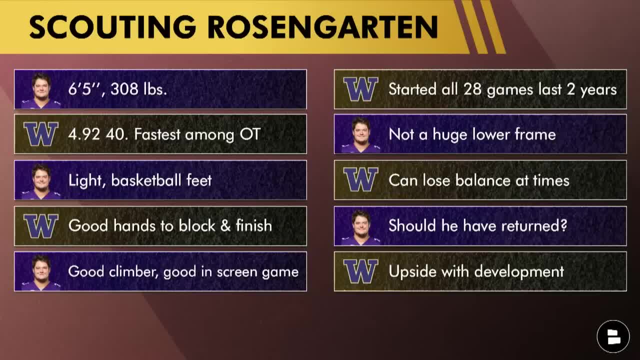 mean by that on some of these full blocks he can get out in space and get to that second and third level on the screen game And obviously Kyle Shanahan likes to do that within his offense. He's been a durable player. Has started all 28 games over the last two years. 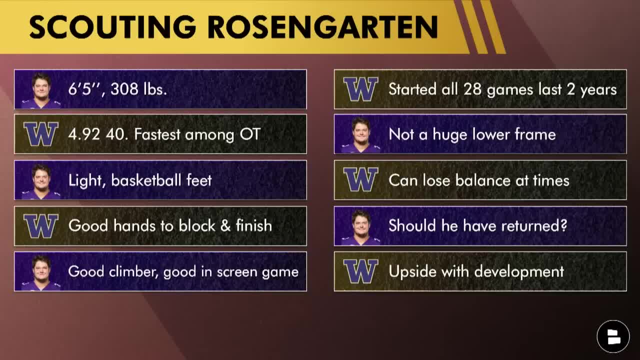 The weaknesses here, not a huge lower frame that can cause him to lose balance at times, that can cause him to get uprooted. And Monk Kuyper said in his previous mock draft that if Rosengarten were to go back to Washington he felt as though he could be a top 10 pick At number 31,. 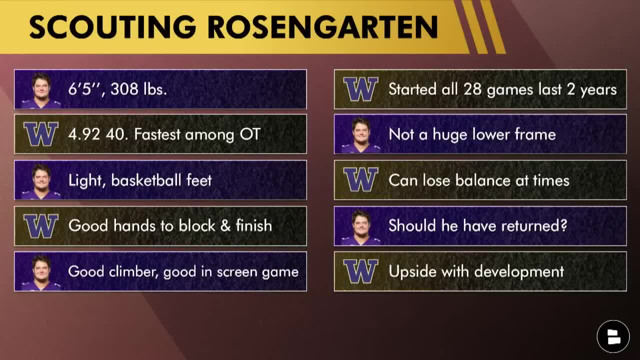 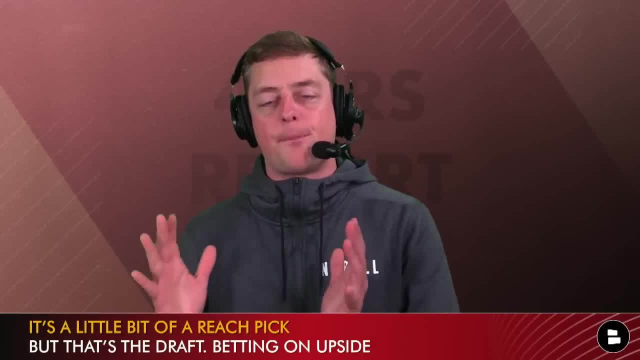 a lot of people think this is a reach because a lot of other NFL draft evaluators think that he should go somewhere in the 50s, 60s, maybe even in the 70s. So developmental project, a little bit of a reach, but that's what the draft is Oftentimes. 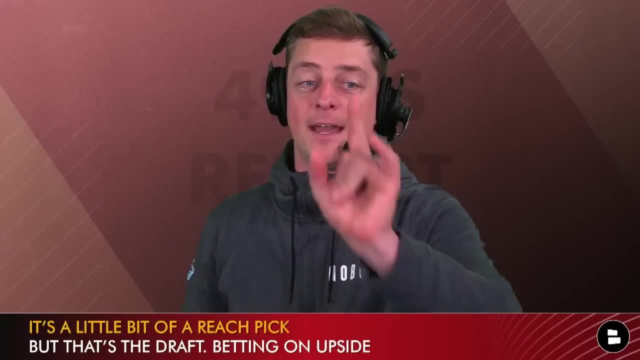 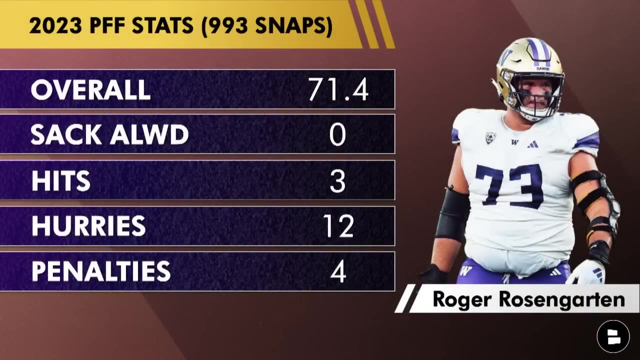 you're betting on upside, And this is what I'll tell you right now. If the Niners draft him, I still think he's better than Colton McKevitt. The pro football focus numbers in 2023, 993 snaps for a Huskies team that made it all the way to the national championship. 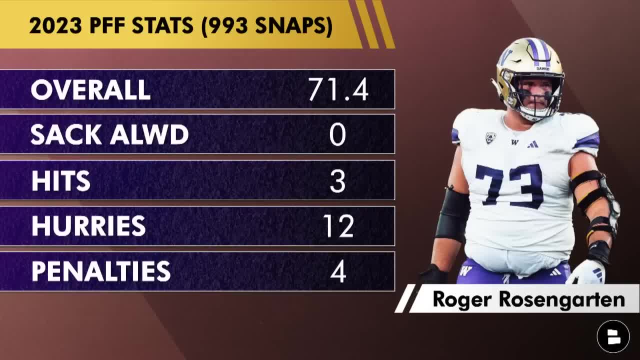 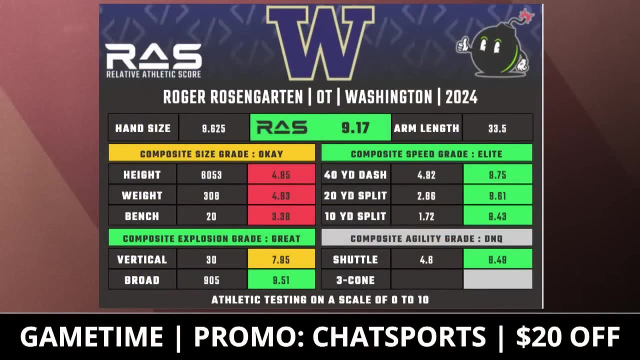 pulled off an epic win over Texas in the college football playoff semifinal. Rosengarten with those, no sacks allowed. 71.4, pro football focus grade, 12 hurries and four penalties. The athletic testing numbers very solid. I don't really get why Math Bomb on the relative athletic score here. 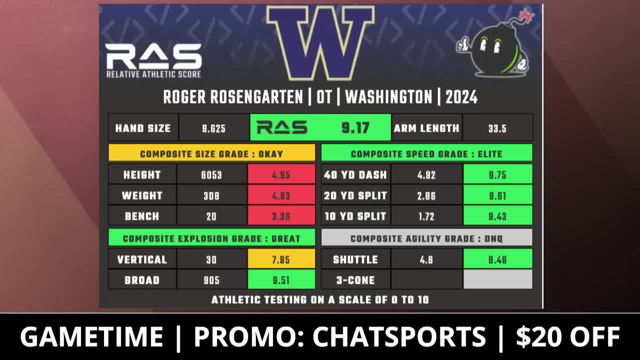 has his height in red. I mean, my dude is 6'5". He is a little bit lighter at 308 pounds, but offensive linemen, who were light and good athletes, you can build on that frame. He did bench 225 pounds 20 times. So sometimes, ideally, you look for offensive. 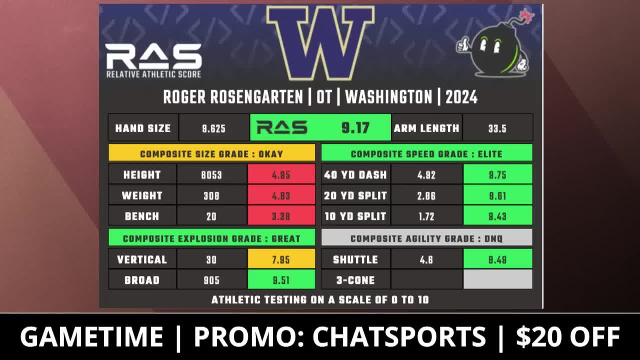 offensive linebackers who are light and good athletes. He did bench 225 pounds 20 times, So to put up 25, 30 reps. but that's not an end-all be-all. At the end of the day his relative athletic score was a 917.. Good broad jump, the 40-yard dash- incredible at that size. 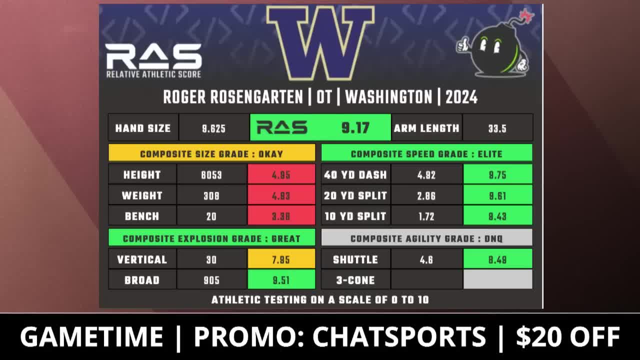 and that short area quickness with the 20-yard split, 10-yard split. It's important for when you drop back in your pass sets but also when you get to that second and third level on some of those run-blocking plays. Are you happy with Mel Kuyper's pick of Roger Rosengarten? 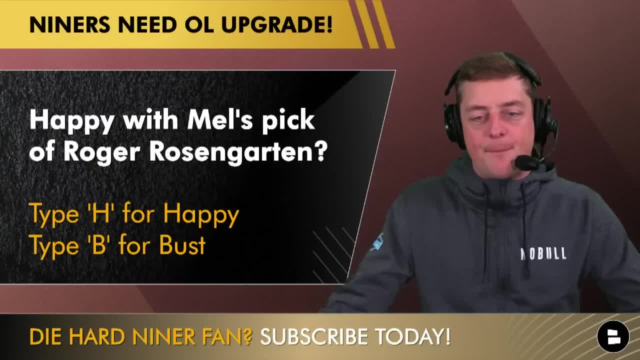 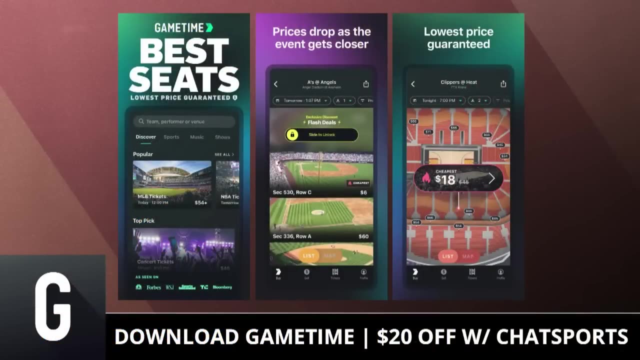 To the Niners at 31,. type H for happy or B for bust. What do you think about who Mel Kuyper has going to the San Francisco 49ers here in his latest mock draft? Today's show is sponsored by GameTime, the only ticketing app that gives you a complete peace of mind with your purchase. 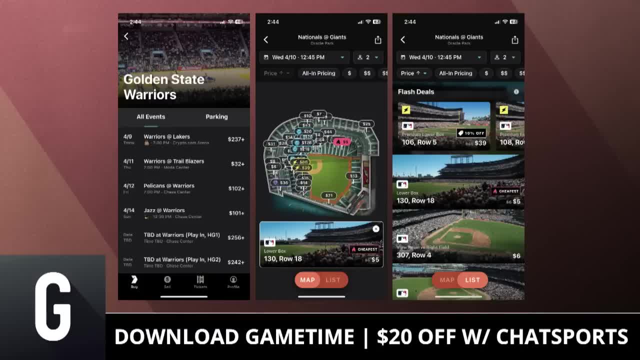 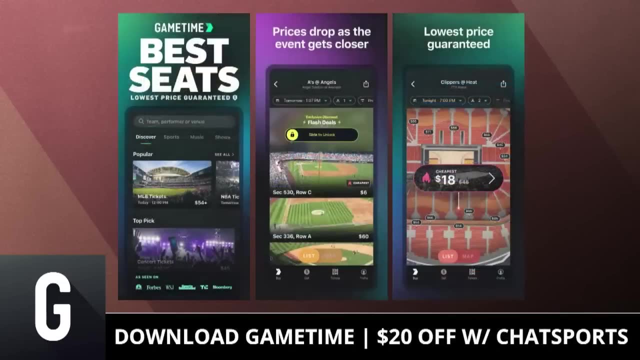 See the view from your seat before you buy, so you know exactly what to expect when you arrive. All-in prices show your total up front, so you know you're getting a great deal. before you check out. Buy tickets in seconds with just two taps. GameTime has deals on tickets right up to the start of any event and even an hour after. 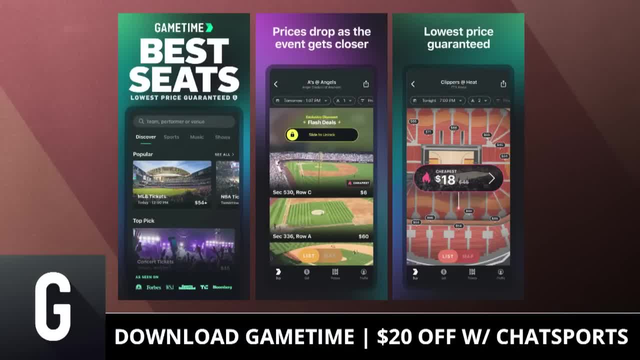 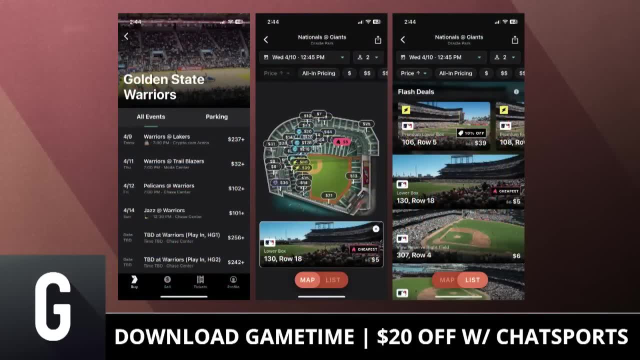 it starts. If you're running a little bit late, you can't make a decision until late in the process. It's the place to find last-minute seats, find exclusive flash deals and sponsored deals on tickets for football, basketball, baseball, concerts, comedy, theater and more, And 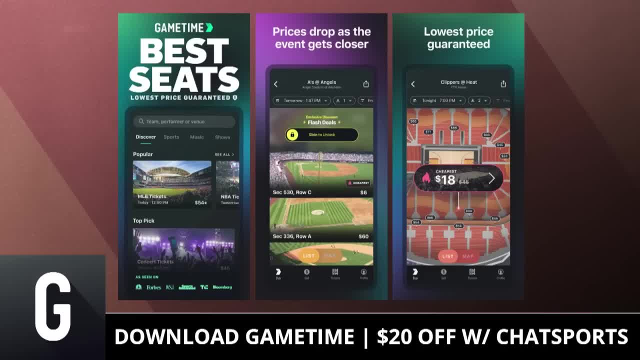 they're exclusive flash deals and sponsored deals on tickets For all of these events. allow you to save money. get in the door at a very affordable price tag. There are also zone deals, too, So download the GameTime app, create an account, use the code. 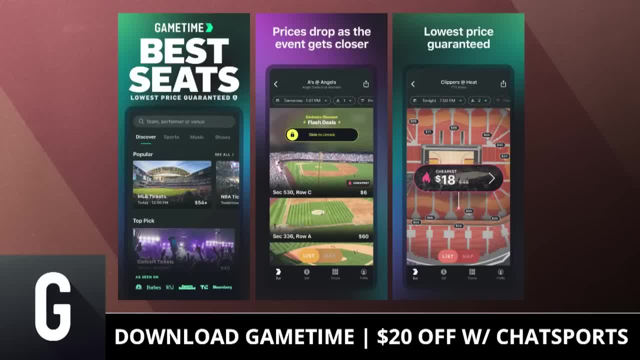 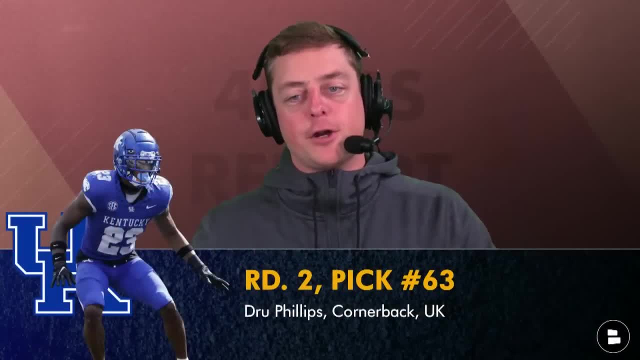 CHATSPORTS for $20 off. your purchase Terms apply. create that account and use the code CHATSPORTS for $20 off. So the Niners go off. it's a tackle: 31st overall pick in Kuyper's draft. 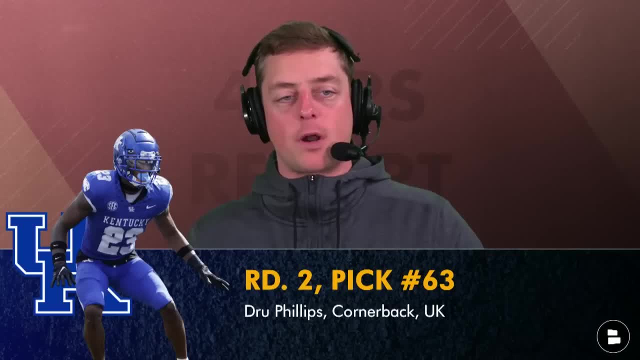 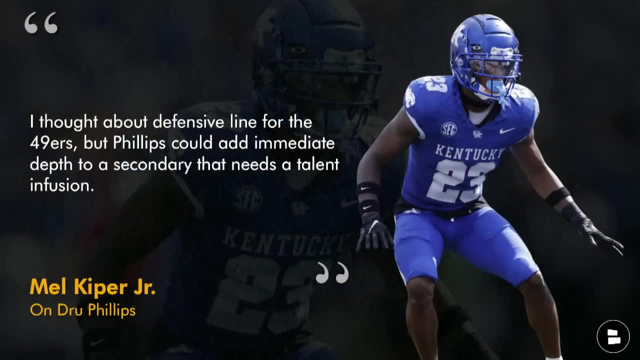 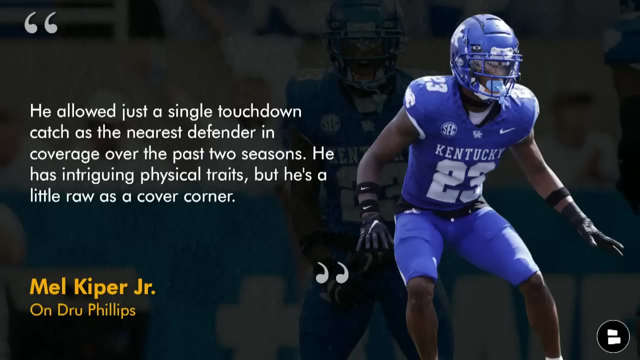 Round two, pick number 63,. they go with Drew Phillips, the quarterback out of Kentucky Kuyper, with the short right up here I thought about defensive line for the Niners, but Phillips could add immediate depth to a secondary that needs a talent infusion. He allowed just a single touchdown catch as the nearest. 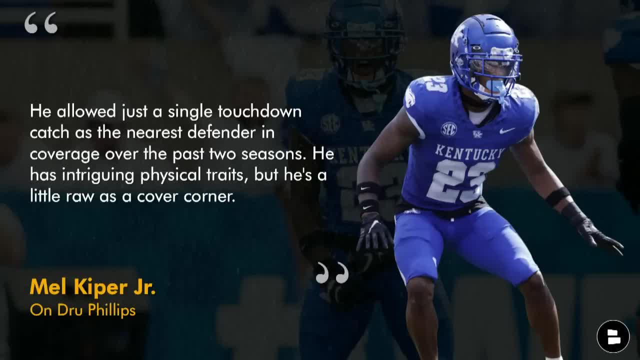 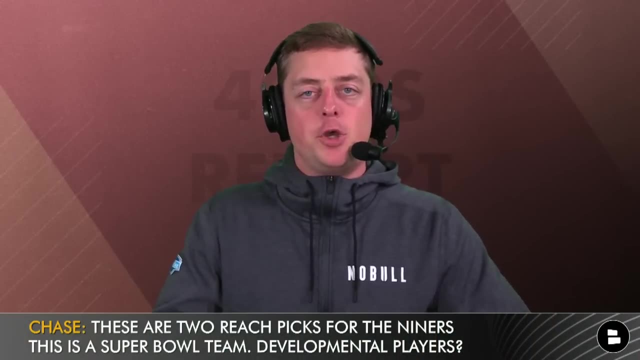 defender in coverage over the last two years playing in the SEC. by the way, He has intriguing physical traits but he's a little robbed as a cover cornerback, I think. for me, up to this point, looking at what Kuyper's done, these are two reach picks for the Niners. You can go better. 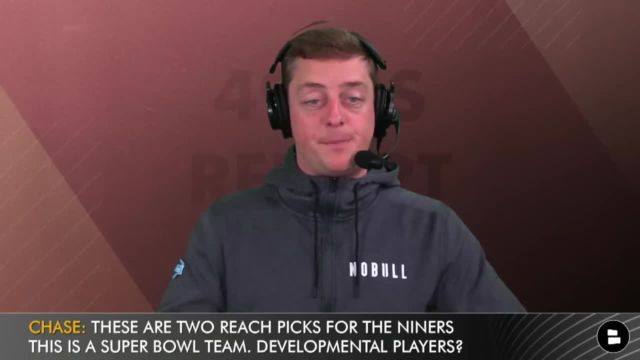 here with best, better players available, also known as BPA, best players available on the draft board. And for the Niners, this is a Super Bowl team that we're talking about and we're drafting developmental players. at this point, When I scout Phillips again, he has upside, He has potential. 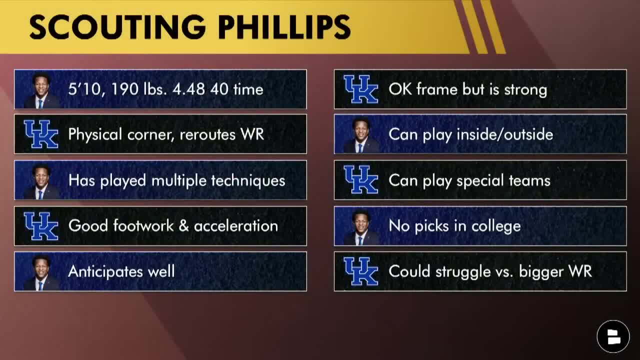 He's 5'10", 190 pounds. a sub 4'5" 40-yard dash. a 4'4" 8" was his best time. He's a physical corner who can reroute wide receivers. He has played multiple techniques. 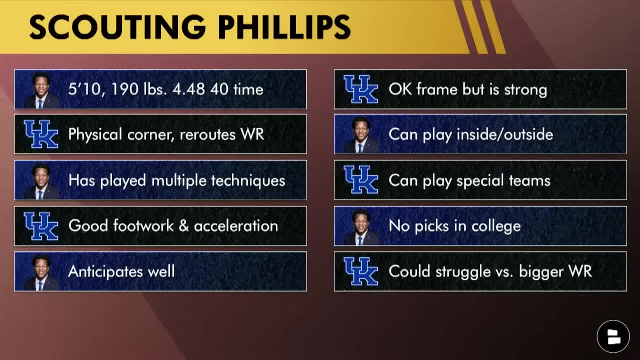 which I'm sure the Niners would really like. He has good footwork and acceleration. I think he anticipates very, very well- and the Niners love corners, who can anticipate an okay frame. but he's strong. He loves hitting the weight room, so you don't have to worry about the 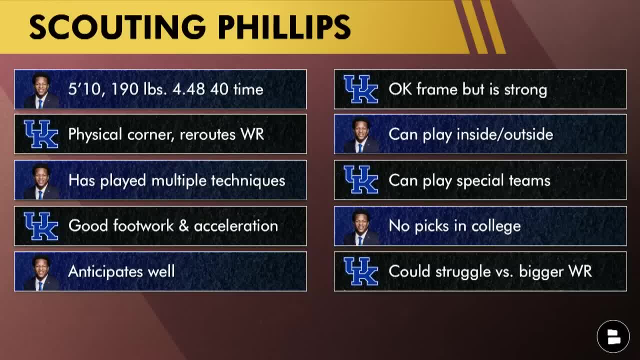 dedication. He has versatility. He could play inside, outside. He played every snap against Tennessee as a slot corner in 2023. He can also play special teams. He had no interceptions in college, which is a little bit weird, and Kuyper threw out the stat of not giving up a. 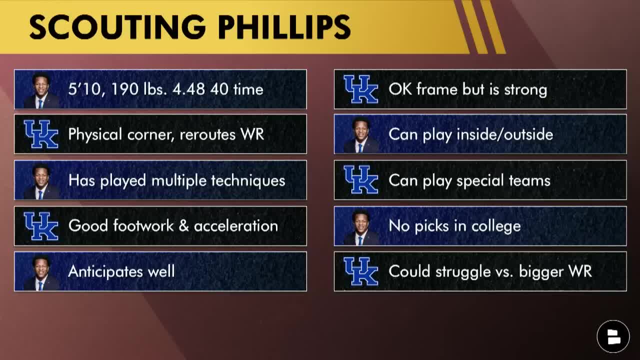 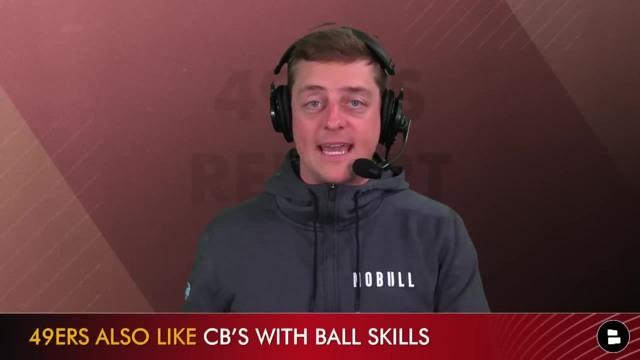 touchdown as the nearest defender. That's great, but no picks. He could struggle because of that frame of 5'10" and not having a lot to build upon as far as that frame against bigger wide receivers at the NFL level. To me this sounds like a slot corner at the NFL level: 5'10". 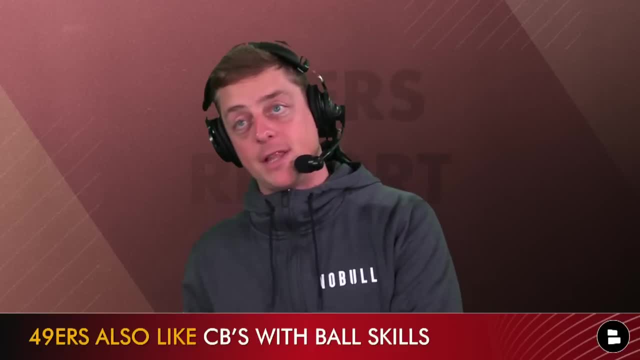 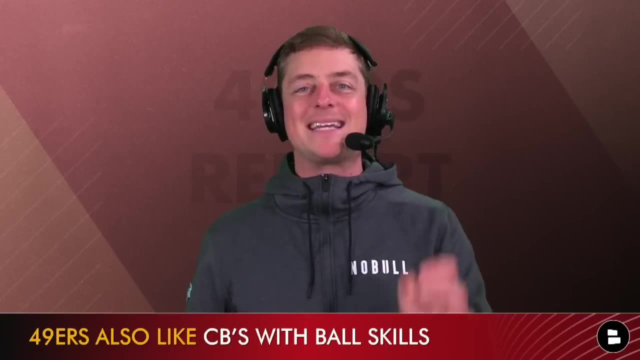 not a big frame. He's tough, doesn't have a lot of interceptions. There's a slot corner on the board here at this point. The player who I'm going with is Mike Sainristill, out of Michigan. The Niners like these corners with ball skills. 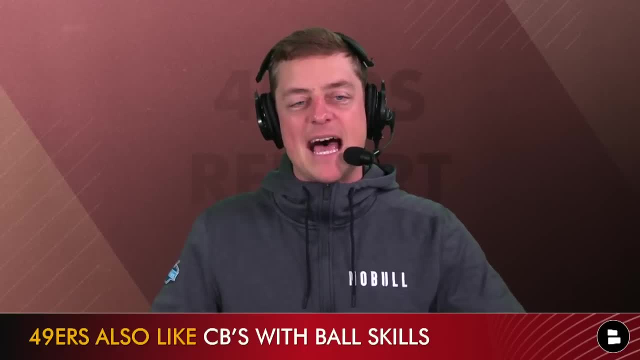 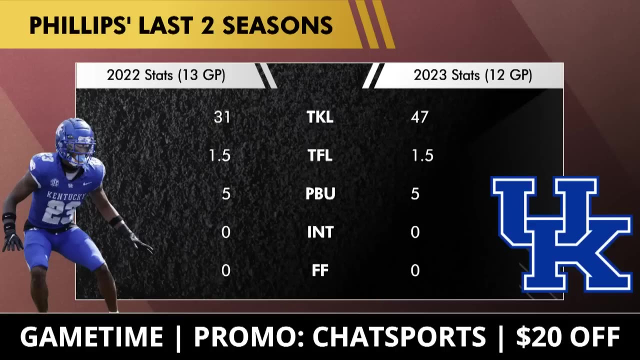 so this could be a player that they decide to target. His last two years, 2022,: 31 tackles, one and a half TFLs, five pass breakups, no picks, no forced fumbles. Obviously, those numbers consistent as far as the INTs and forced fumbles the last two years, as you can see.